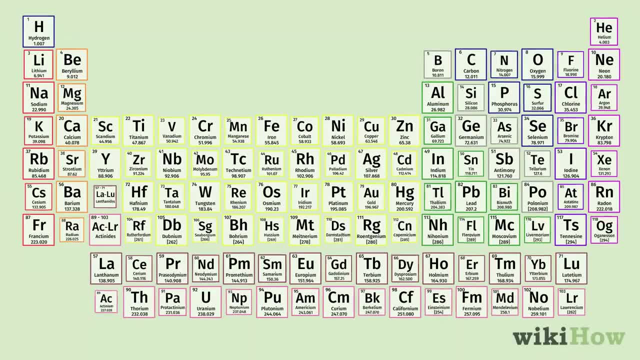 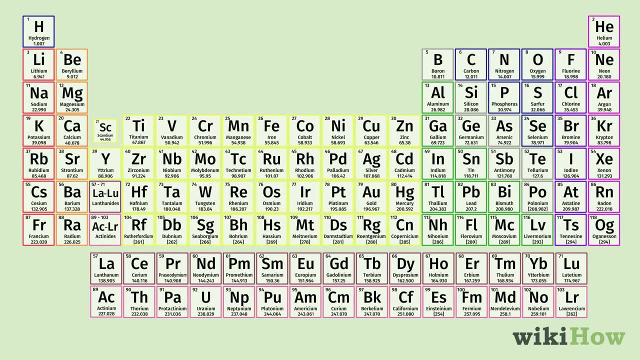 The periodic table can seem a little daunting at first, but it's not too difficult to understand once you learn the basics of how it works. When you're reading the periodic table, move across the table from top left to bottom right. As you move across the table, the number of protons and the atomic mass of each element, 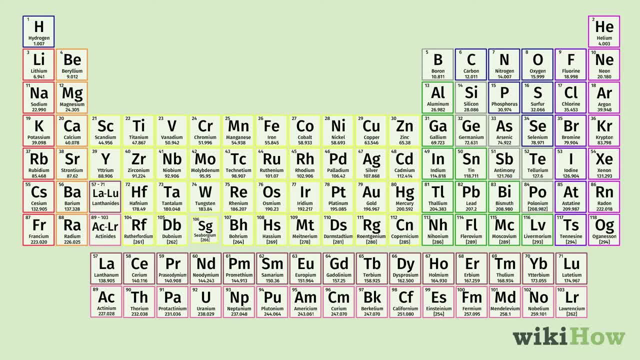 increases. Each element has its own atomic number, which represents the number of protons in one atom of the element. For instance, the first element in the periodic table, hydrogen, has an atomic number of one, because a hydrogen atom has only one proton. 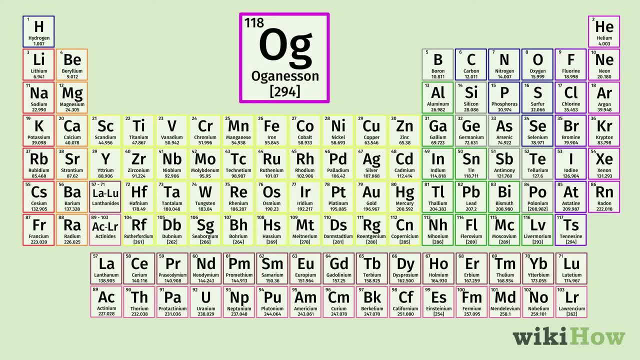 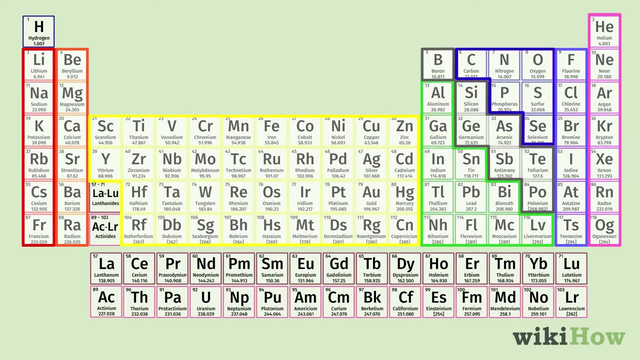 At the other extreme, an atom of the synthetic element, organicin, has 118 protons and an atomic number of 118. The elements are all atomic. The elements are also organized into groups or families that share similar physical and chemical properties. 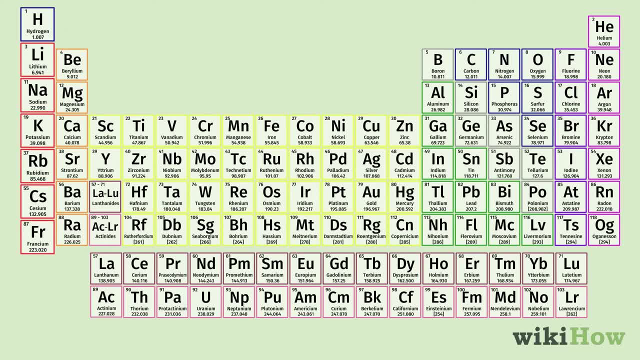 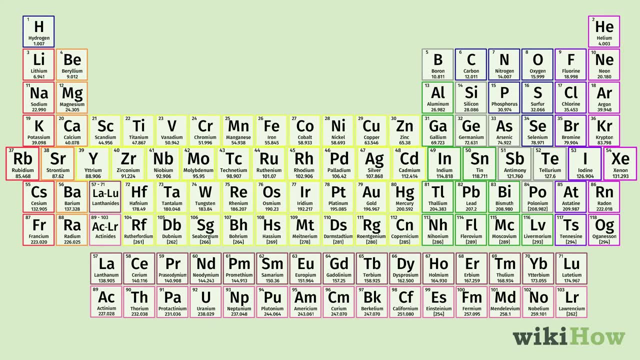 Each column in the periodic table going from top to bottom represents one of these groups. Additionally related elements are usually color-coded to indicate whether they are metals, semi-metals or non-metals. When you read the periodic table in rows going across from left to right, you will find that 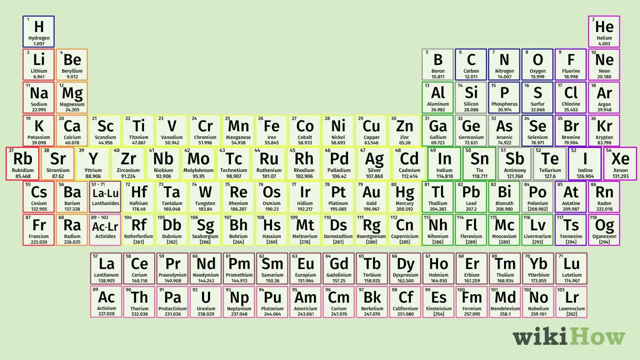 the elements in each row share the same number of atoms. The elements are also organized into groups or families that share similar physical and chemical properties. In the briefly presented example, we have three atomic orbitals. The orbitals are the regions around the atom's nucleus where electrons are most likely to 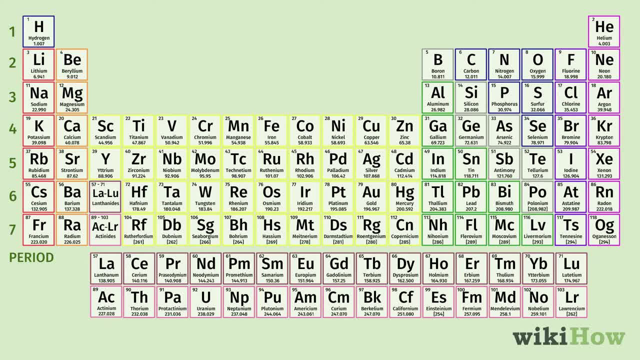 appear. Each of these seven rows is called a period. Finally, you might notice that there are gaps in the periodic table, particularly in the top three rows. This is because the elements don't always fit neatly into groups that share the same physical and chemical characteristics. 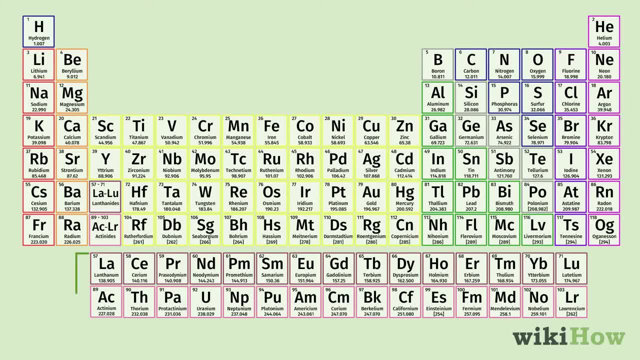 The elements are one group of elements that have nearly independent components. The elements in a group are not grouped into a single group. Therefore, there are some elements that are not grouped together And some elements are not grouped together. indistinguishable chemical properties, called the rare earth's elements, is separated out into its 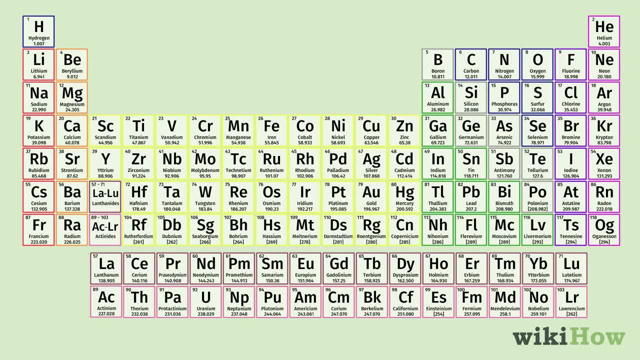 own separate space at the bottom of the periodic table. When you look at individual elements on the periodic table, there are several pieces of information that you can find on each square. For example, every element has a one- to three-letter symbol that represents the name.